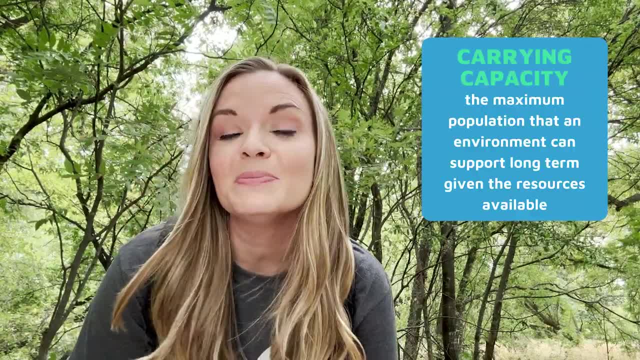 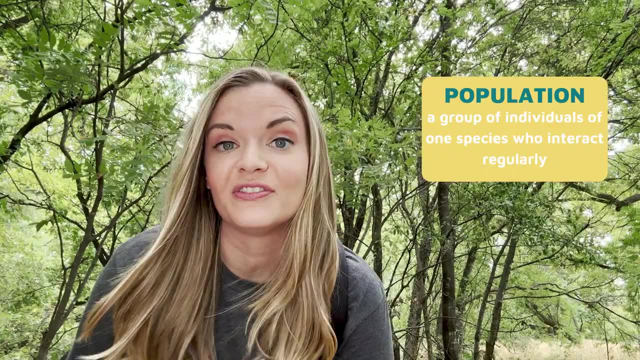 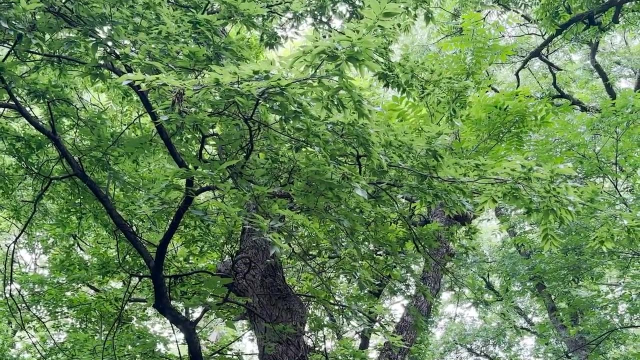 environment. The carrying capacity of an environment is the maximum population that environment can sustain long term with the resources available. A population is a group of individuals of the same species who interact regularly. So our squirrels here on the nature trail are a population. 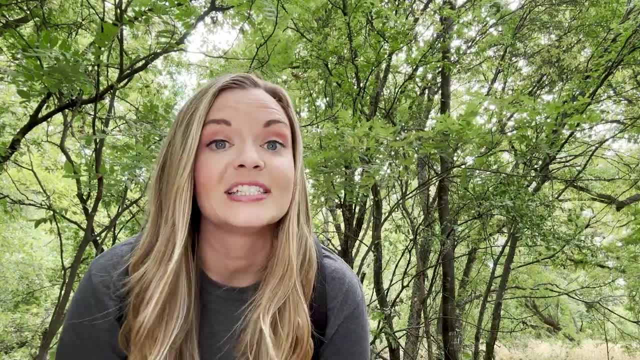 The resources we're talking about are the resources we're talking about here. The resources we're talking about here are the resources we're talking about here. The resources we're talking about here are the things that an organism needs to live and reproduce. These resources vary for different species. 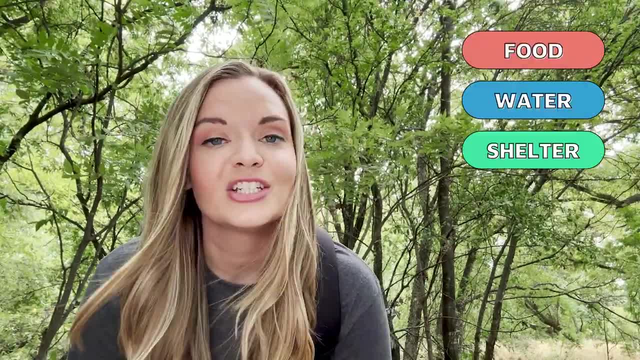 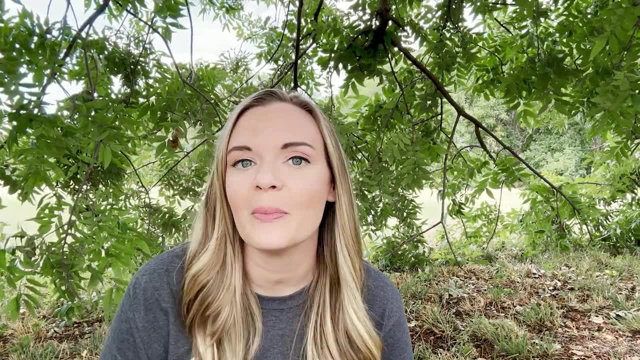 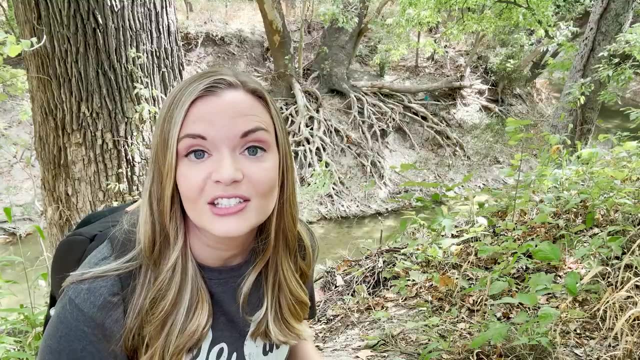 but are mostly things like food, water, shelter and space For our squirrel friends. this nature trail ecosystem that we're in has a higher carrying capacity than, say, a city block. The trail follows this creek. that provides plenty of water. There are even tons of. 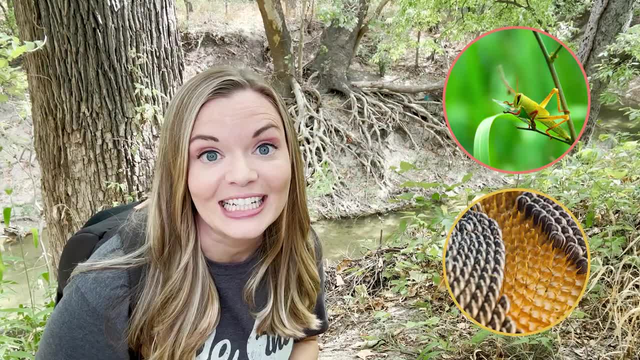 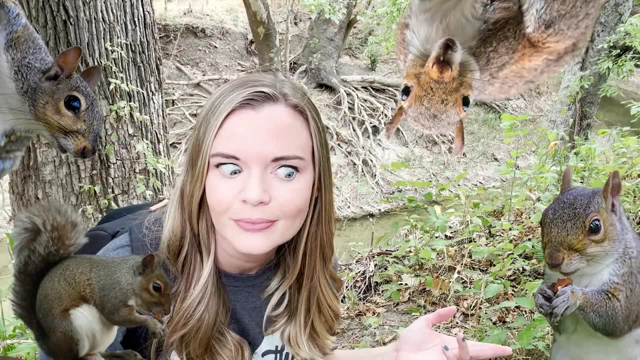 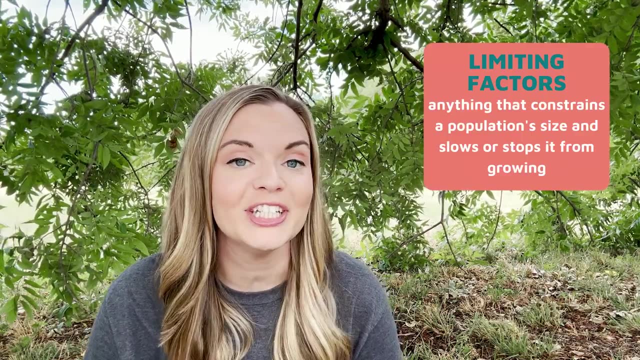 grasshoppers and seeds, like sunflower seeds, for them to eat. The population is strong here, so why aren't there hundreds of squirrels running all over the place? Because, even though there are tons of resources here, there are limiting factors that are keeping the squirrel population in check. 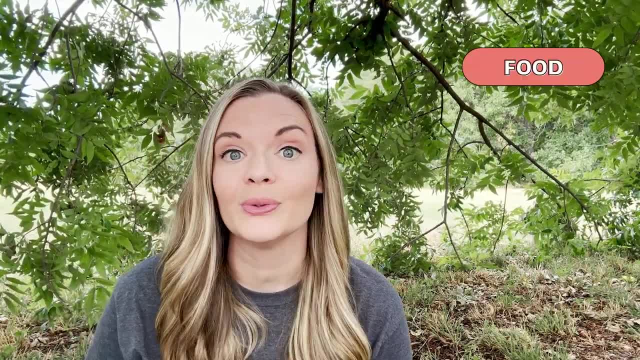 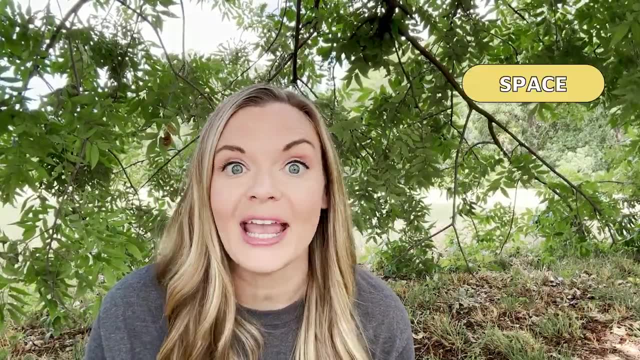 We have already covered a few limiting factors like food, water and shelter. Not enough of those, and your population will decline. But what about things like space and predation? Squirrels aren't territorial like bears or lions would be, but they do need space for. 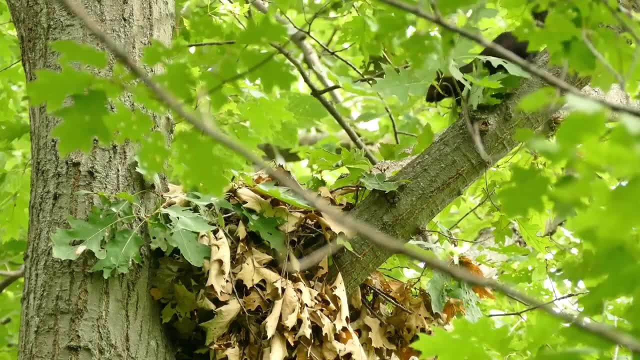 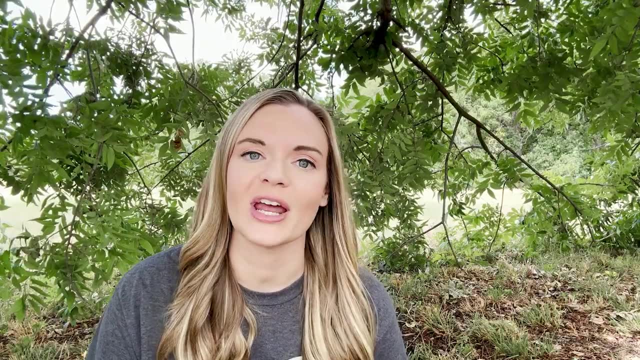 their nests And they do not like other squirrels getting close to their babies. So if nesting space is limited, it could force some squirrels out of this area. Squirrels' main predators are birds of prey animals like redtail hawks. 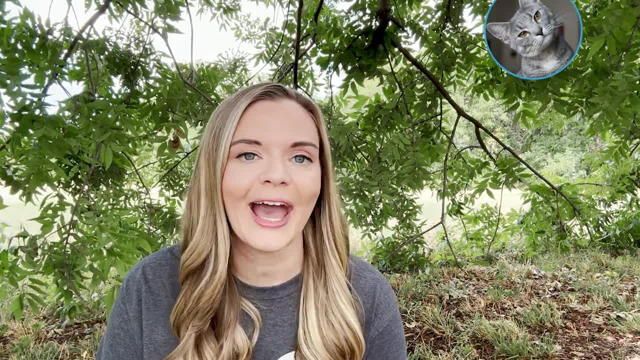 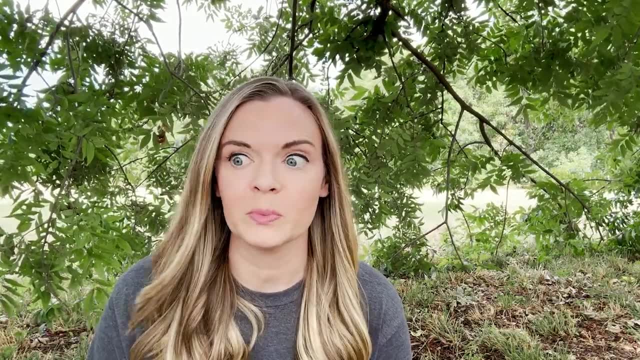 kites and owls, But they can also fall prey to cats, dogs, snakes and raccoons, especially when they're young. Predation limits the population. The more squirrels an ecosystem has, the more predators it can sustain In this. In this area there is a family of kites that I see all the time and I can hear calling to each other when I'm out on the trail. I have also seen several snake species that would absolutely eat a young squirrel like this copperhead. 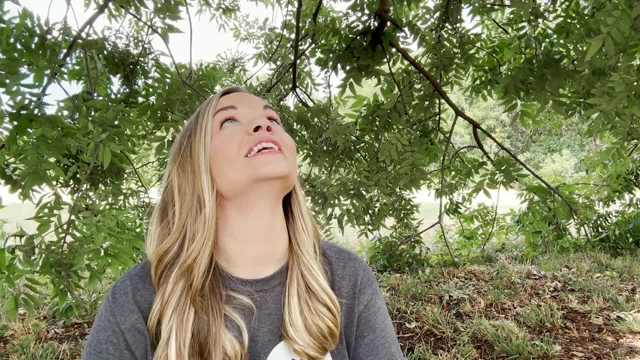 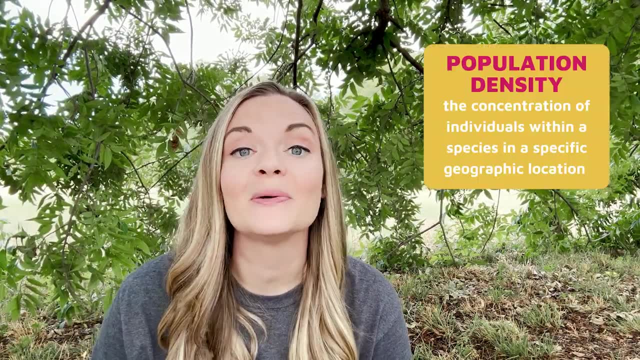 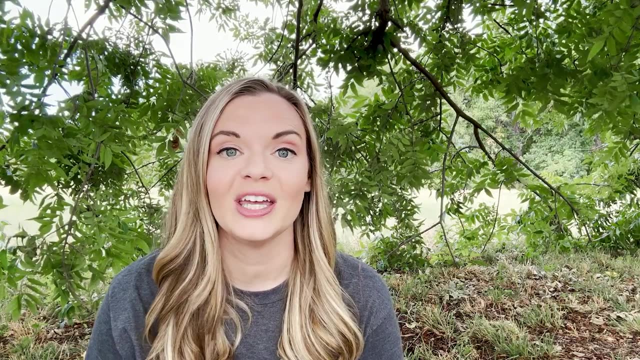 Hi, little chickadees, Don't poop on my head. The number of squirrels in this specific area is the population density. It's the number of individuals divided by the size of the area. The population density changes when individuals are born or die, move into the area or leave. 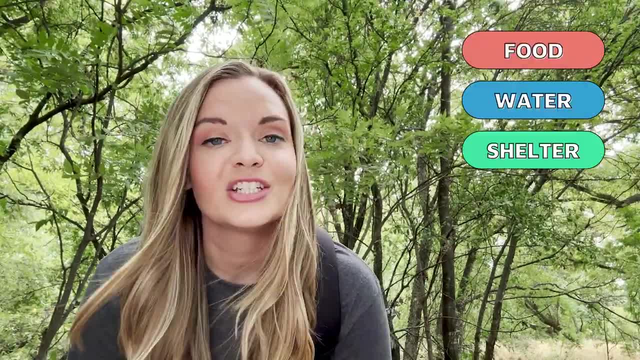 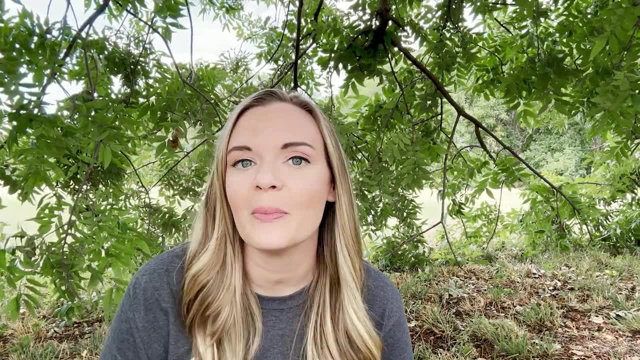 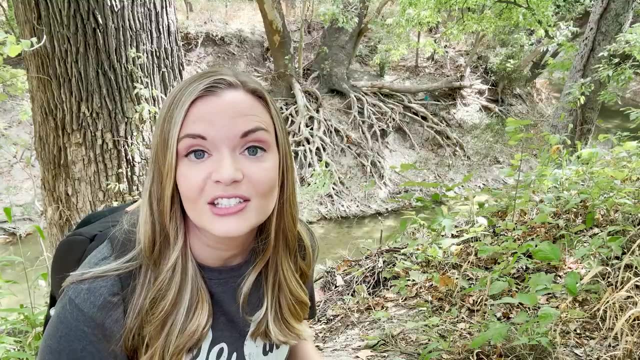 but are mostly things like food, water, shelter and space For our squirrel friends. this nature trail ecosystem that we're in has a higher carrying capacity than, say, a city block. The trail follows this creek. that provides plenty of water. There are even tons of. 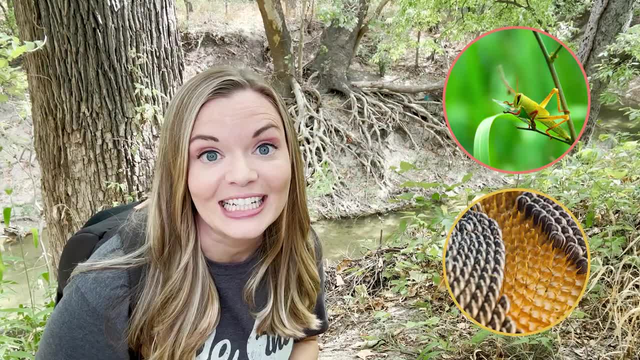 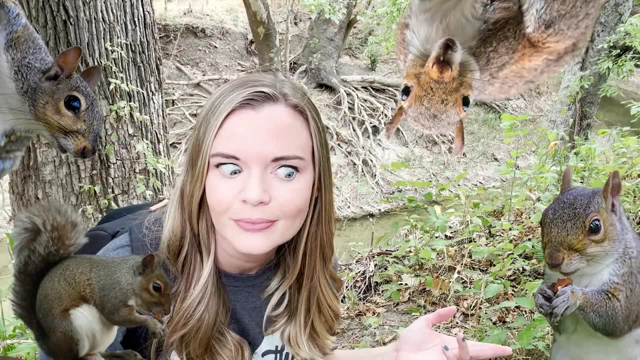 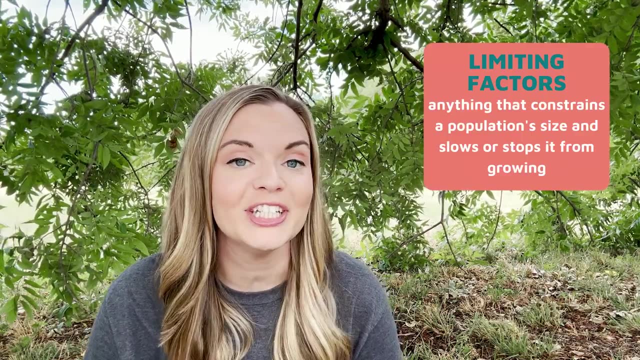 grasshoppers and seeds, like sunflower seeds, for them to eat. The population is strong here, so why aren't there hundreds of squirrels running all over the place? Because, even though there are tons of resources here, there are limiting factors that are keeping the squirrel population in check. 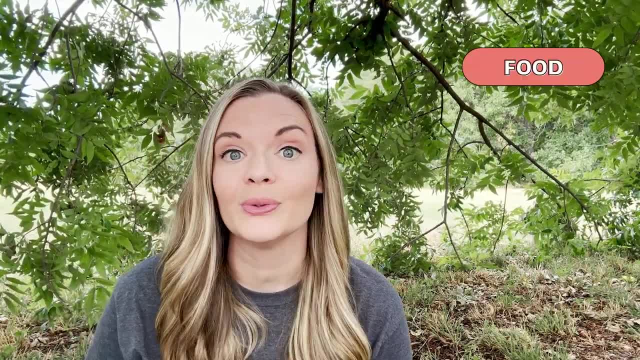 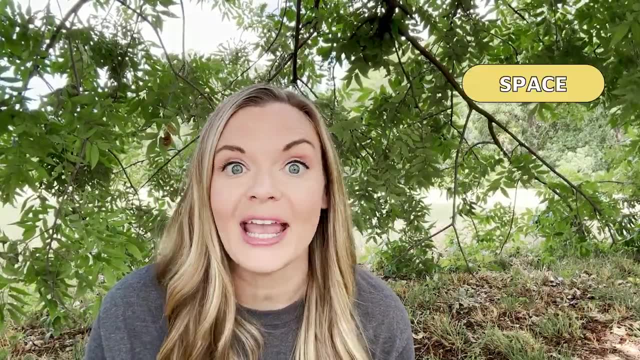 We have already covered a few limiting factors like food, water and shelter. Not enough of those, and your population will decline. But what about things like space and predation? Squirrels aren't territorial like bears or lions would be, but they do need space for. 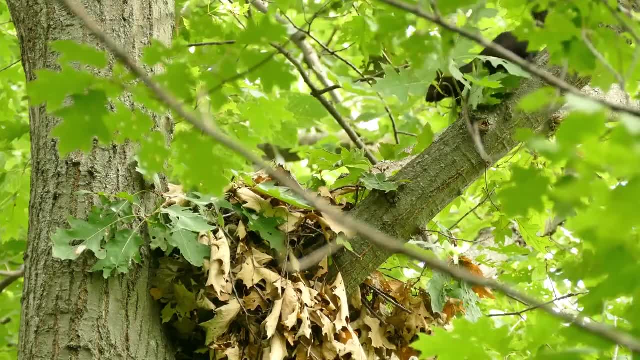 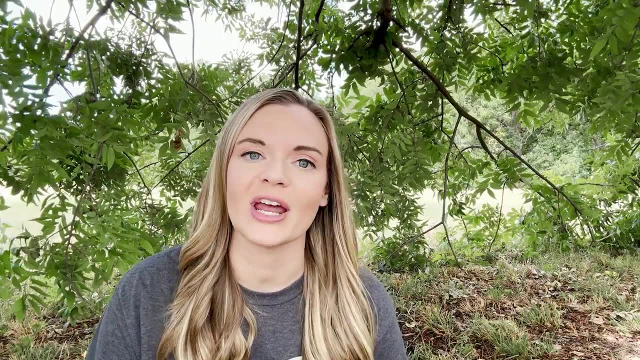 their nests And they do not like other squirrels getting close to their babies. So if nesting space is limited, it could force some squirrels out of this area. Squirrels' main predators are birds of prey, Animals like red-tailed hawks, kites and owls. 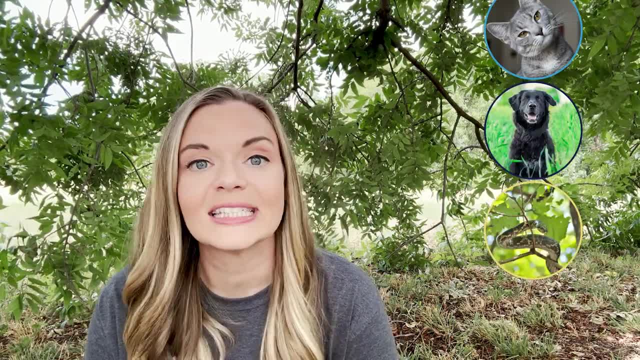 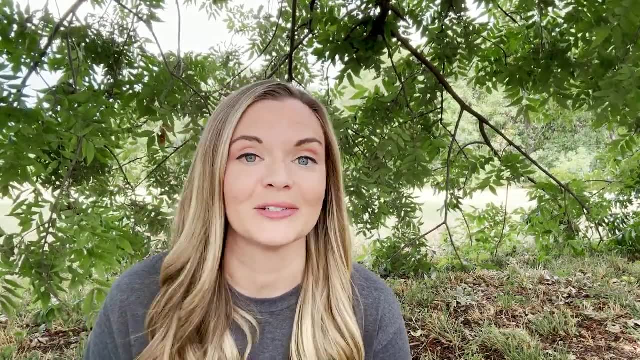 But they can also fall prey to cats, dogs, snakes and raccoons, especially when they're young. Predation limits the population. The more squirrels an ecosystem has, the more predators it can sustain. In this area there are many different kinds of animals and 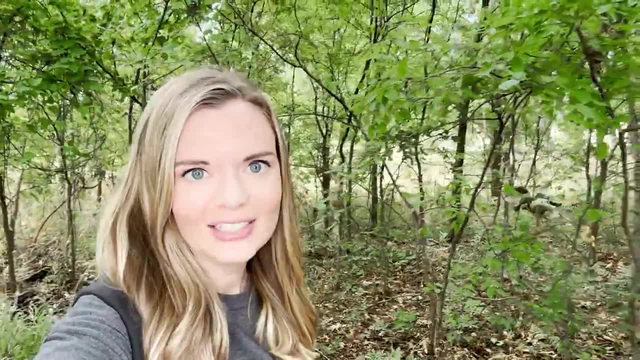 animals that can survive for themselves. In the region of Oregon there are a number of zoos and there are dogs and there's many species of animals that can survive for themselves, But they're not the same species area. there is a family of kites that I see all the time and I can hear calling to each. 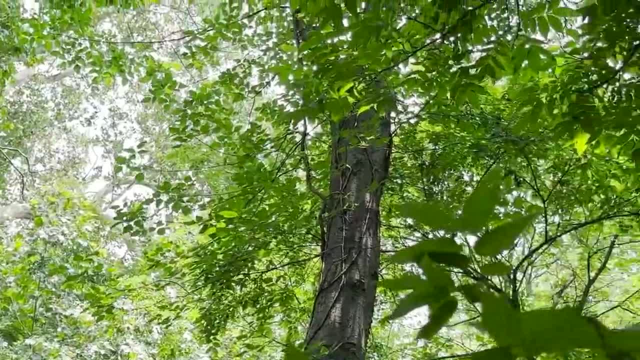 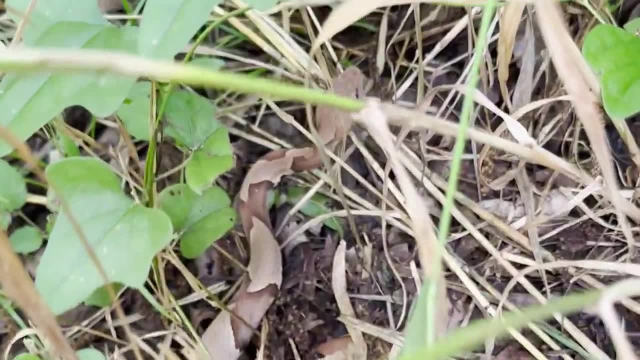 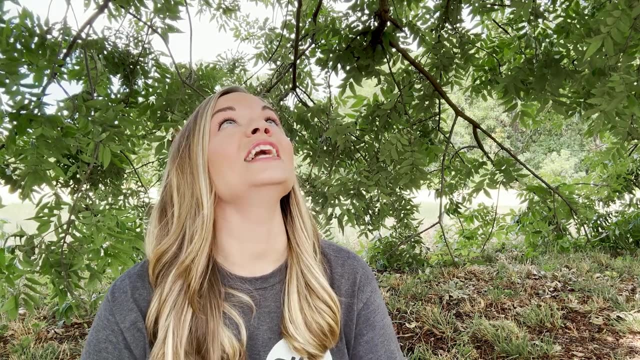 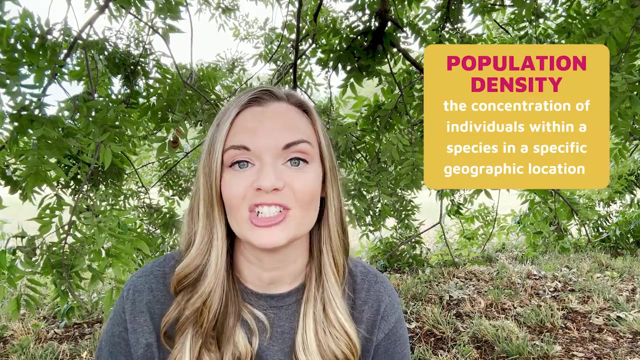 other. when I'm out on the trail, I have also seen several snake species that would absolutely eat a young squirrel like this copperhead. Hi, little chickadees, Don't poop on my head. The number of squirrels in this specific area is the population density. 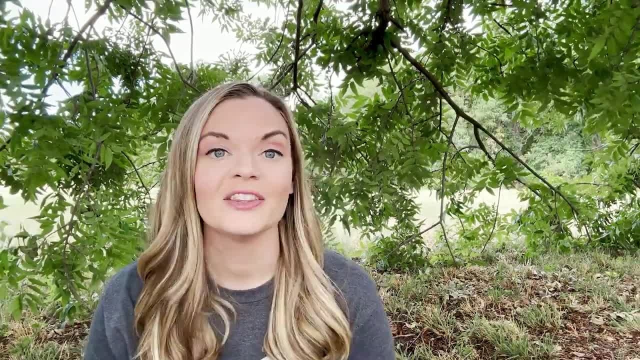 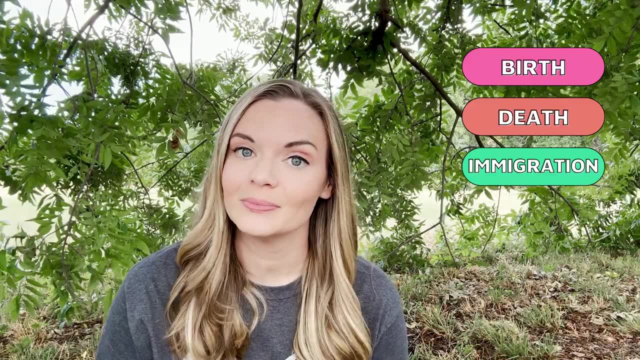 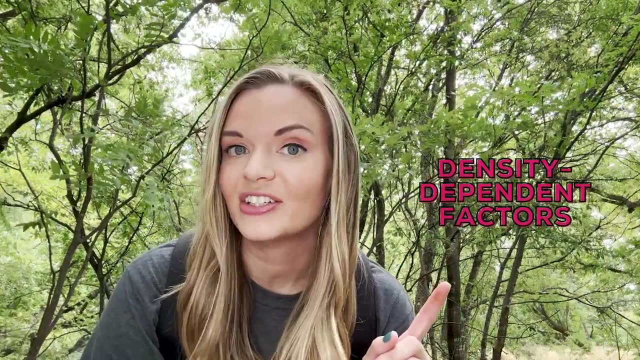 It's the number of individuals divided by the size of the area. The population density changes when individuals are born or die, move into the area or leave the area. The limiting factors that we talked about earlier can be broken down into two types – density-dependent factors and density-independent factors. 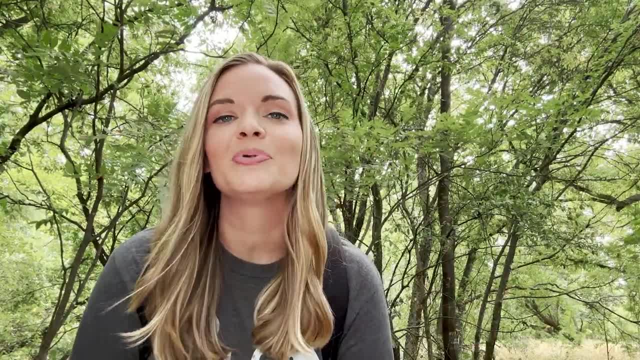 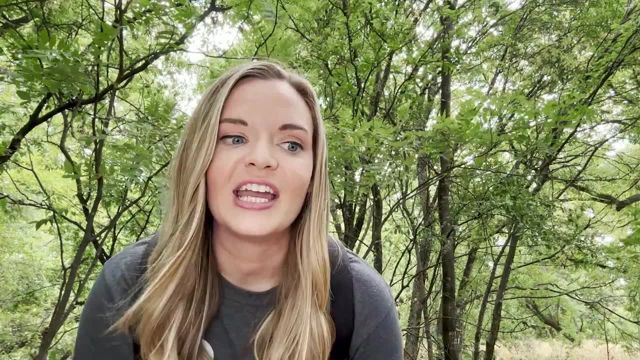 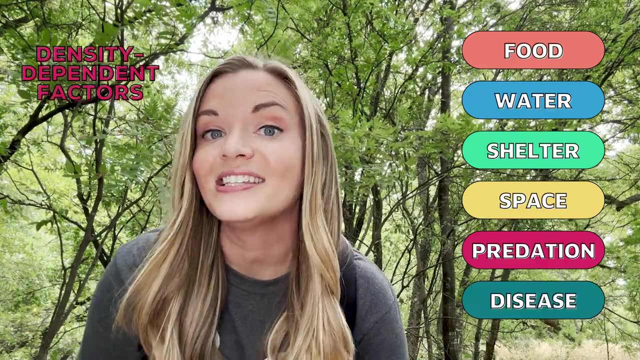 the area. The limiting factors that we talked about earlier can be broken down into two types – density-dependent factors and density-independent factors, Things like food, water, shelter, space, predation and even life. Often things like disease are density-dependent factors. 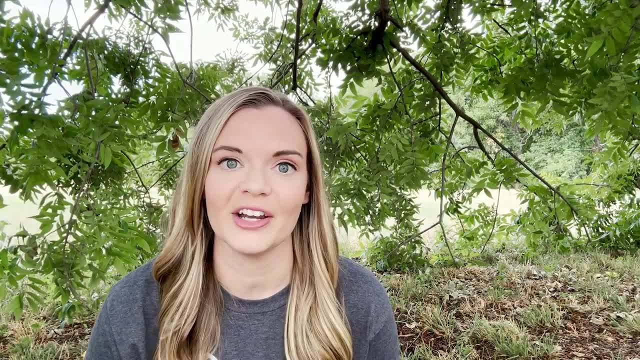 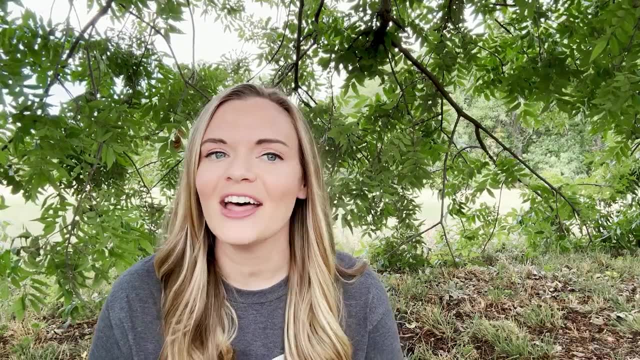 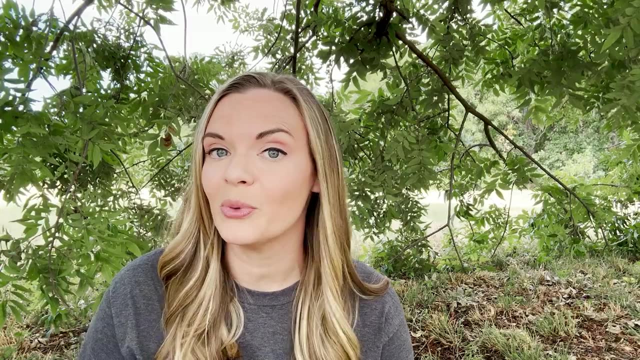 If this area was impacted by something like a wildfire and the squirrels fled to escape the danger, that would be a density-independent factor. The fire has nothing to do with how many squirrels were here to begin with, but absolutely limits the amount of squirrels the area can support after the fire comes through. 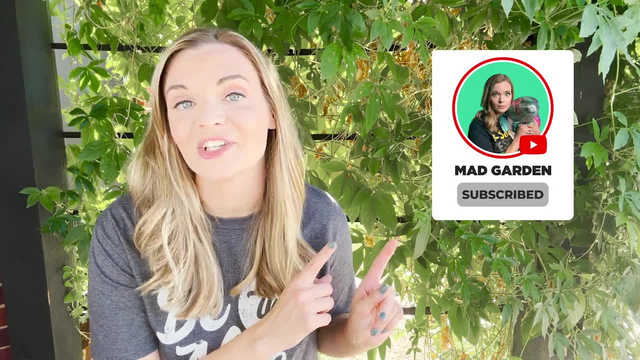 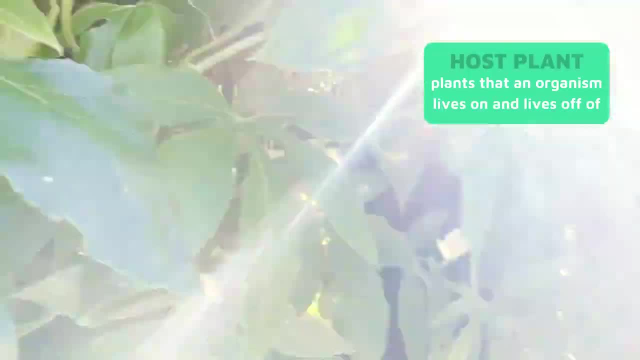 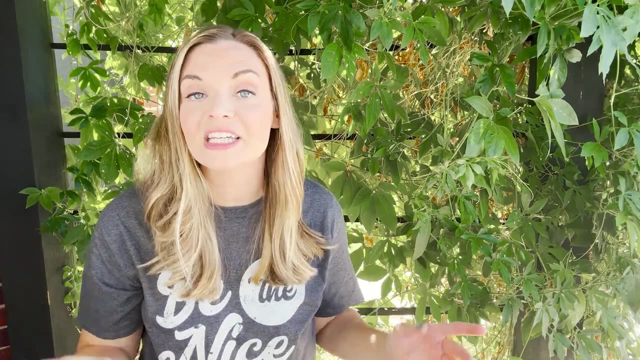 If you're still here liking this video, hit that subscribe button so you never miss an episode. What about another example? This is passion vine. It's the host plant to a species of butterfly called the gulf fritillary. There is a population of butterflies that lives in this neighborhood because this plant 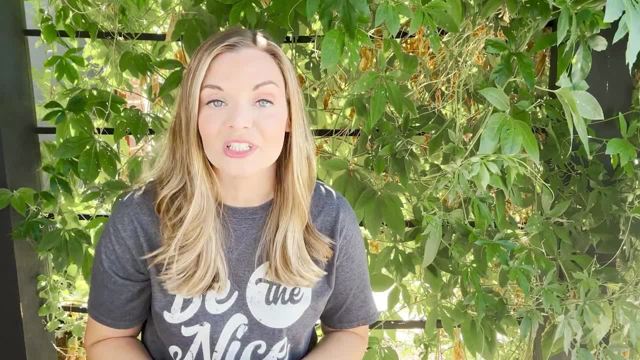 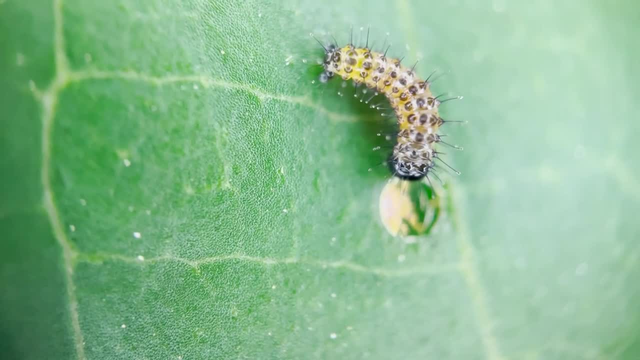 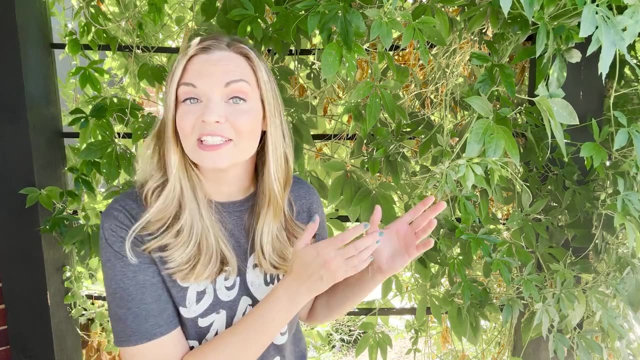 is here In most seasons. the chief limiting factor to this butterfly population is the passion vine itself. Butterflies lay so many eggs that the population grows exponentially. Tons of caterpillars means tons of butterflies. Then those butterflies mate. They lay their eggs back on this same passion vine. 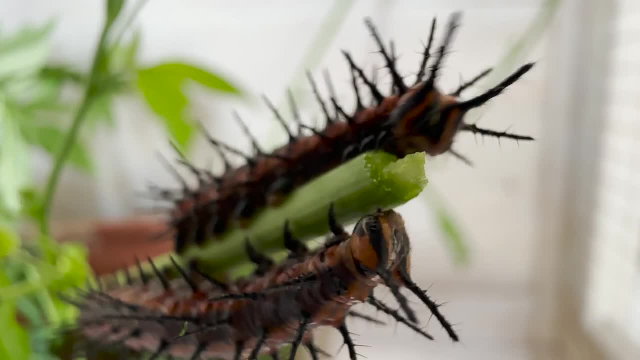 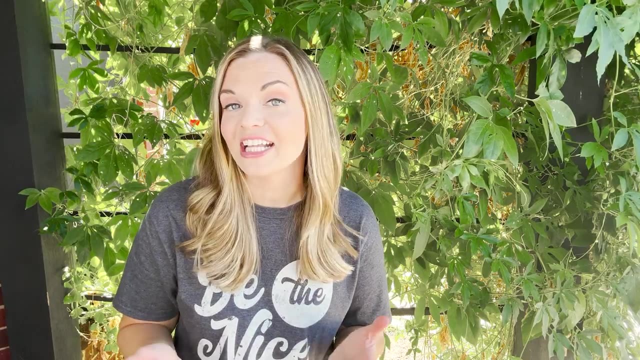 Once the population grows to a certain level, the caterpillars can eat almost every leaf, leaving it looking like a skeleton vine. When the leaves run out, the caterpillars no longer have anything to eat and they will die before they reach their pupa phase. 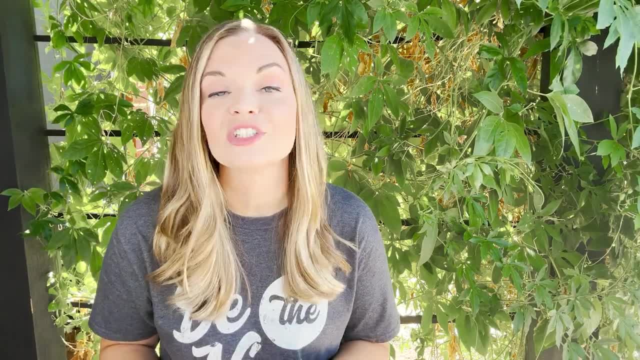 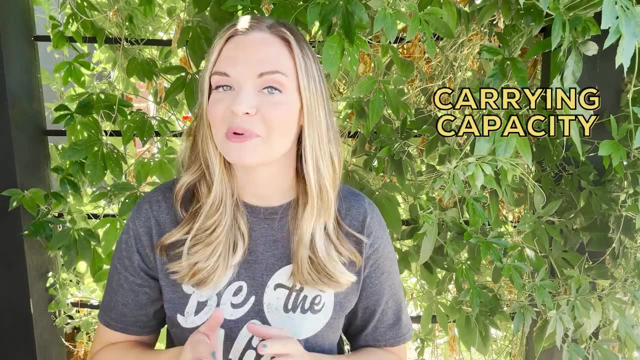 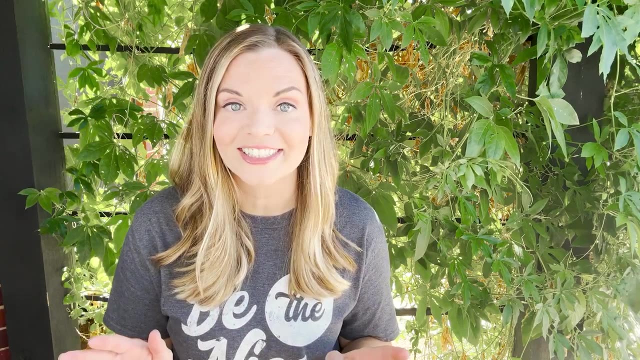 The vine is a fast-growing plant and will bud new leaves to support the next generation. But this population will have reached its carrying capacity, the amount of individual caterpillars it can support with the given resources. This year that same initial growth occurred and there were lots of caterpillars. 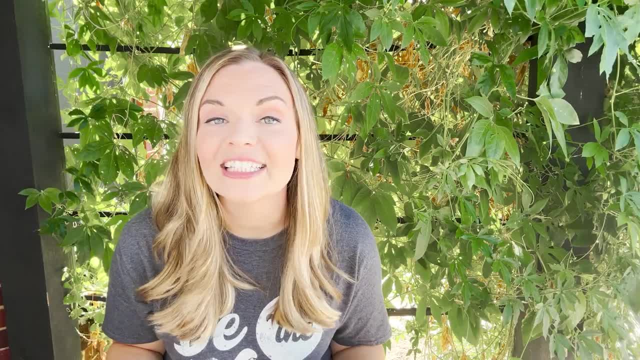 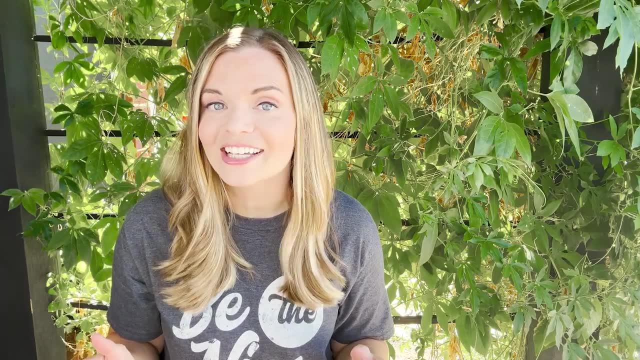 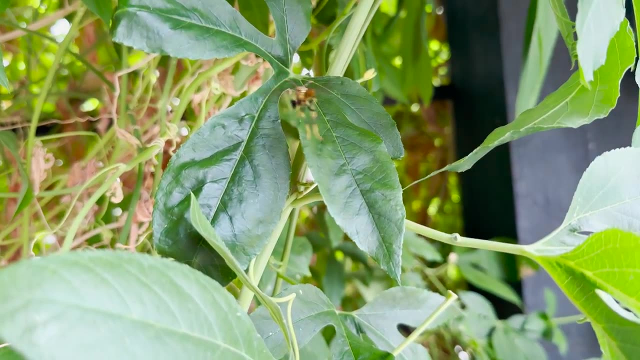 But now the leaves are just covered in holes. The carrying capacity is being greatly impacted by a predator, the yellowjacket. Once the host plant became covered in butterfly eggs, it attracted the predators. Yellowjackets search for butterfly eggs and caterpillars to consume and even destroy. 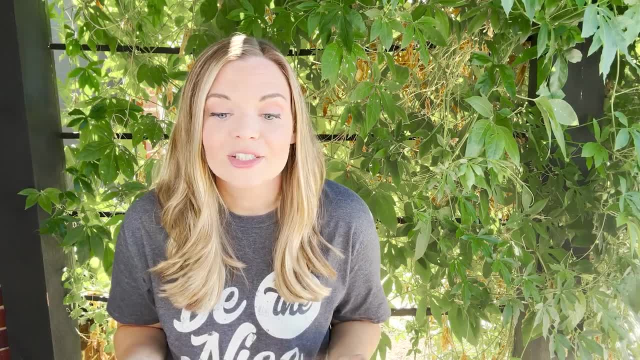 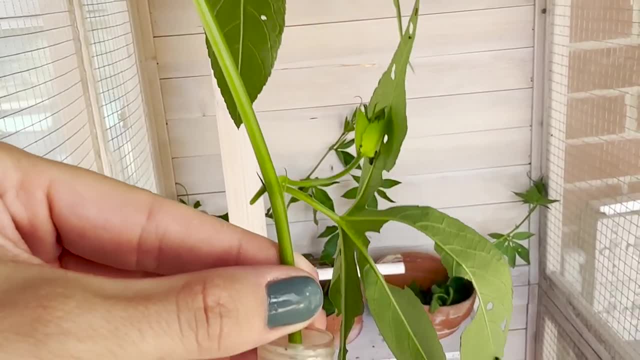 the protective chrysalis. I love these butterflies so I decided to become a factor in their environment. I've started this channel because I love butterflies. I've started collecting the butterfly eggs and tiny caterpillars and moved them right next door to this screened enclosure. 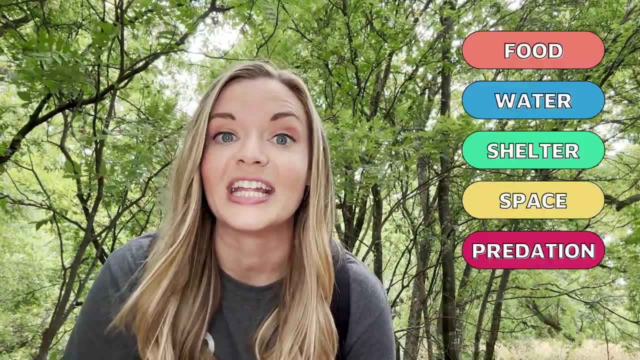 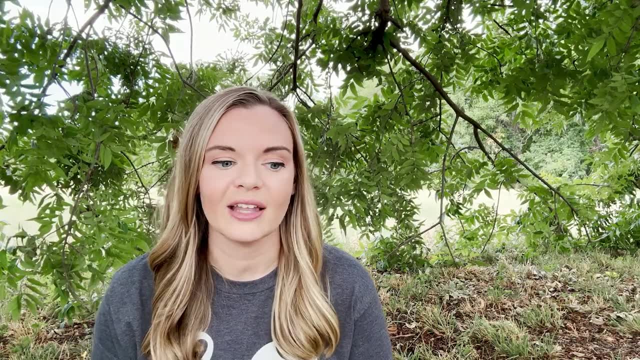 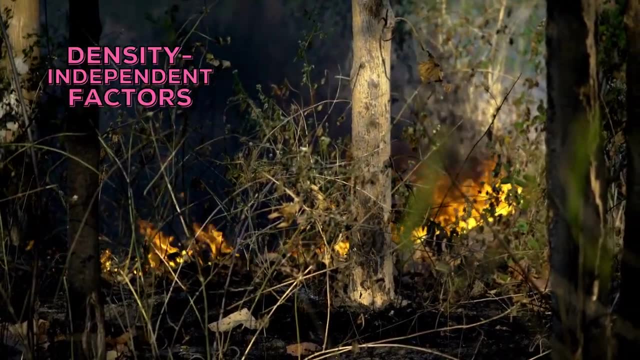 Things like food, water, shelter, space, predation and even life. Often things like disease, are density-dependent factors. If this area was impacted by something like a wildfire and the squirrels fled to escape the danger, that would be a density-independent factor. 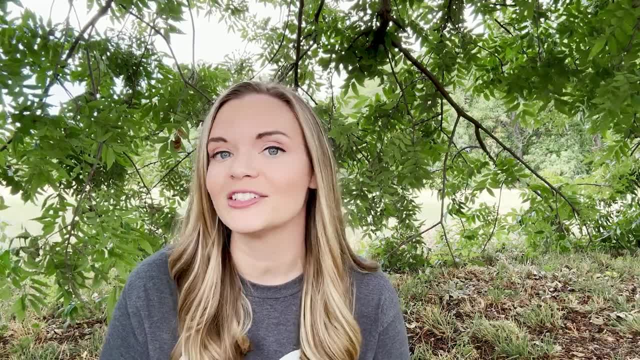 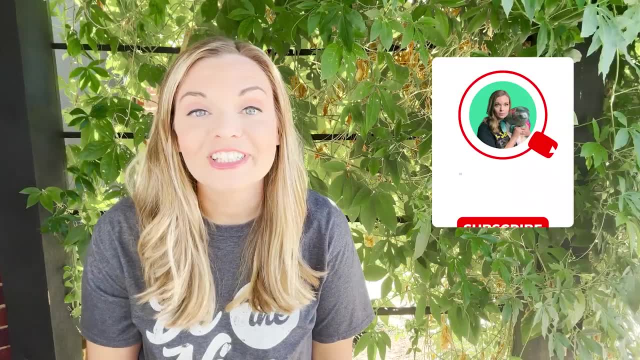 The fire has nothing to do with how many squirrels were here to begin with, but absolutely limits the amount of squirrels the area can support after the fire comes through. If you're still here liking this video, hit that subscribe button so you never miss. 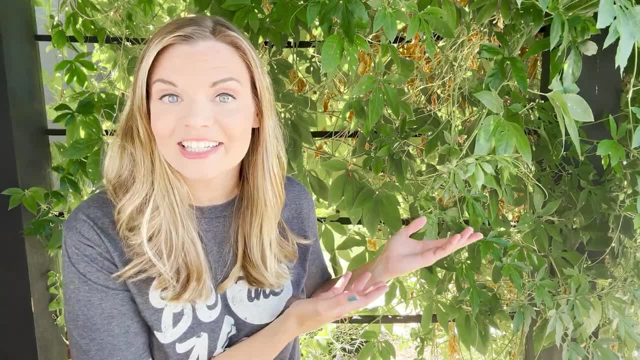 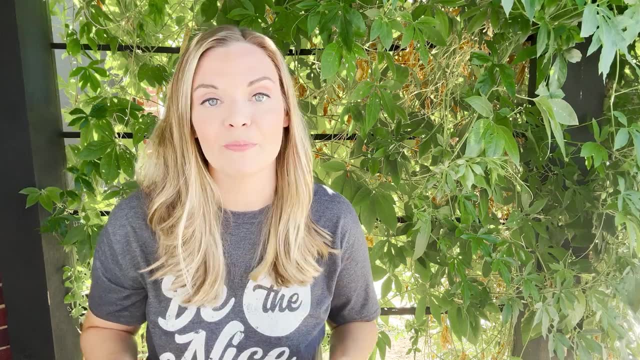 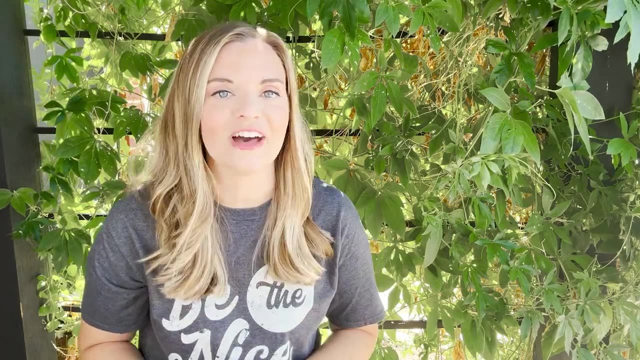 an episode. What about another example? This is passion vine. It's the host plant to a species of butterfly called the gulf fritillary. There is a population of butterflies that lives in this neighborhood because this plant is here In most seasons. the chief limiting factor to this butterfly population is the passion. 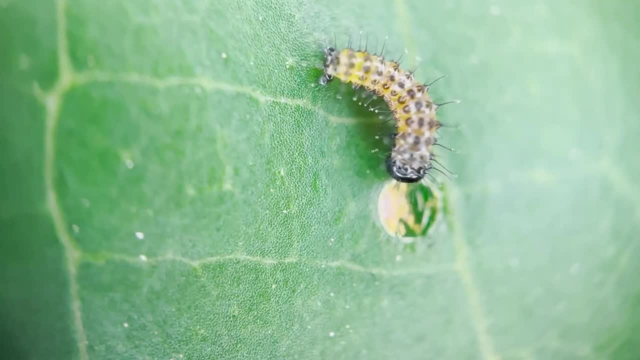 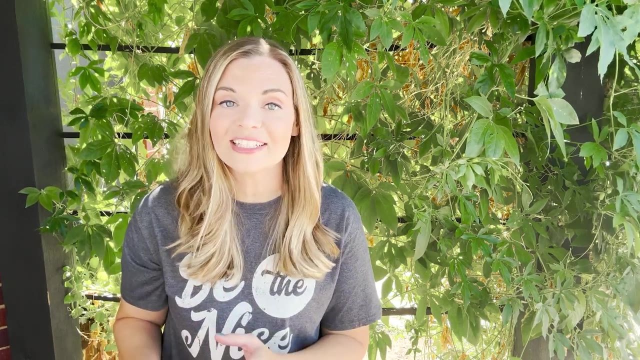 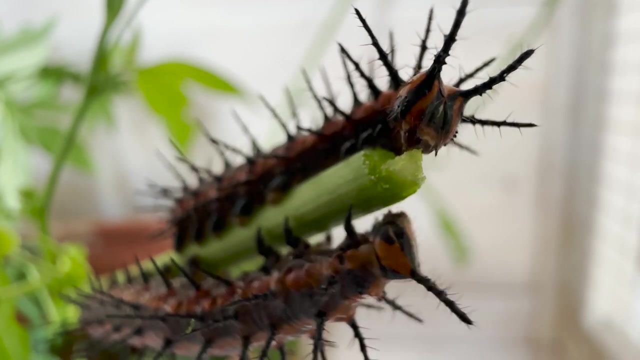 vine itself. Butterflies lay so many eggs that the population grows exponentially. Tons of caterpillars means tons of butterflies. then those butterflies mate and lay their eggs back on the same passion vine. Once the population grows to a certain level, the caterpillars can eat almost every leaf. 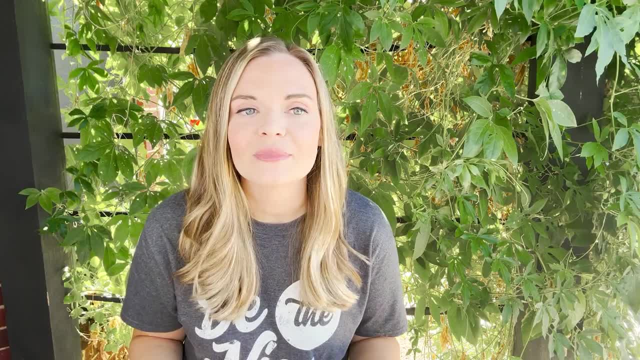 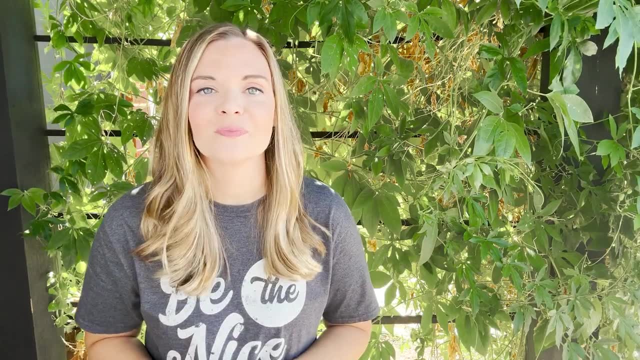 leaving it looking like a skeleton vine. When the leaves run out, the caterpillars no longer have anything to eat and they will die before they reach their pupa phase. The vine is a fast-growing plant and will bud new leaves to support the next generation. 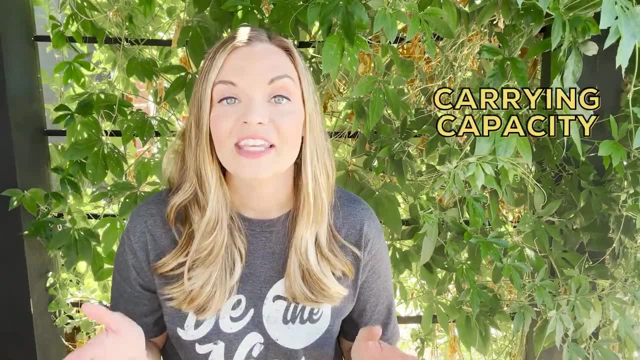 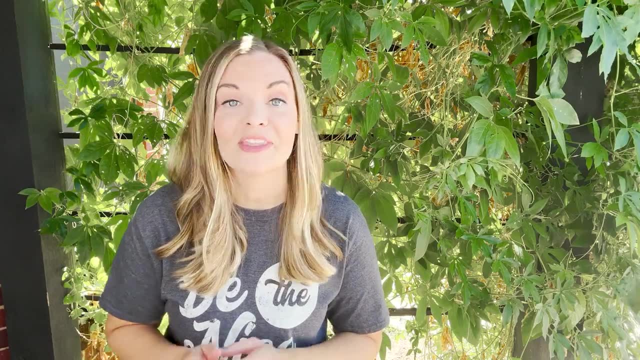 But this population will have reached its carrying capacity- the amount of individual caterpillars it can support with the given resources. This year the population has grown so much that they can't even eat. Last year that same initial growth occurred and there were lots of caterpillars. 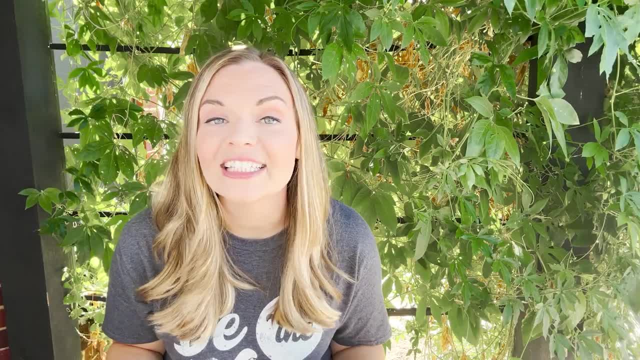 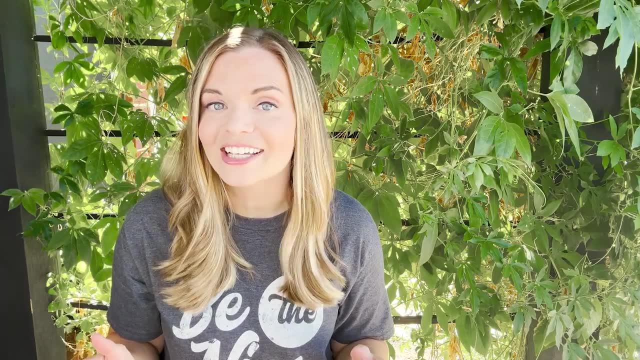 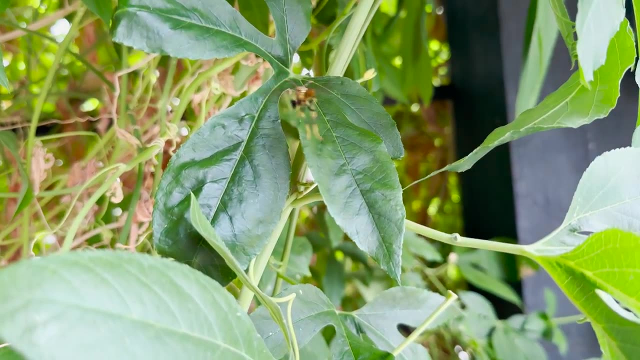 But now the leaves are just covered in holes. The carrying capacity is being greatly impacted by a predator, the yellow jacket. Once the host plant became covered in butterfly eggs, it attracted the predators. Yellow jackets search for butterfly eggs and caterpillars to consume and even destroy. 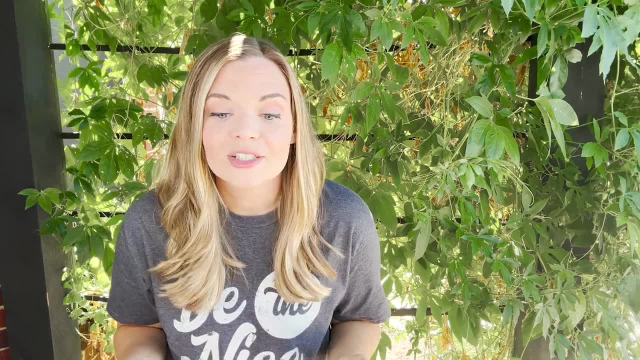 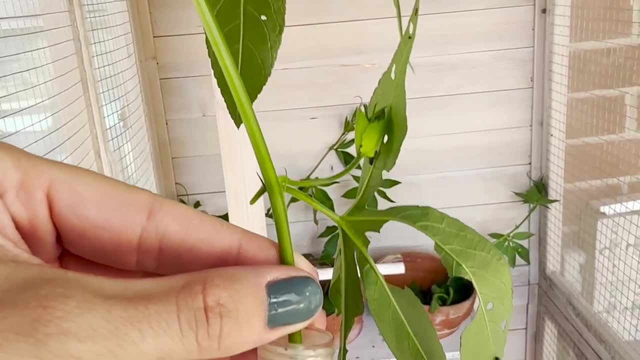 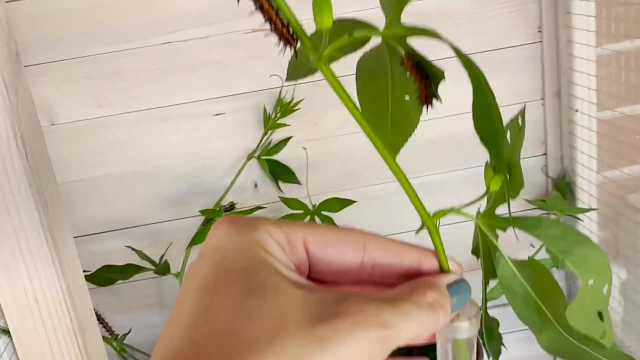 the protective chrysalis. I love these butterflies so I decided to become a factor in their environment. I've started collecting the butterfly eggs and tiny caterpillars and moved them right next door to this screened enclosure. The caterpillars grow happily, eating the leaves of the passion vine I place inside.